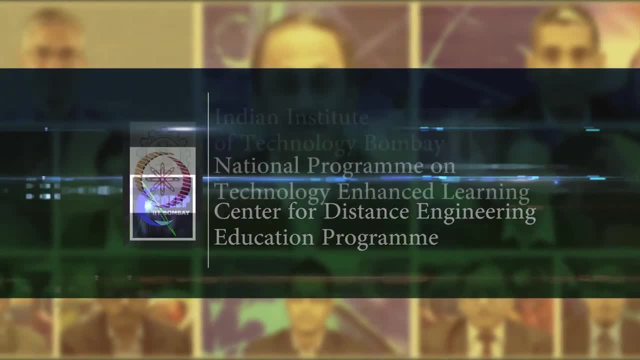 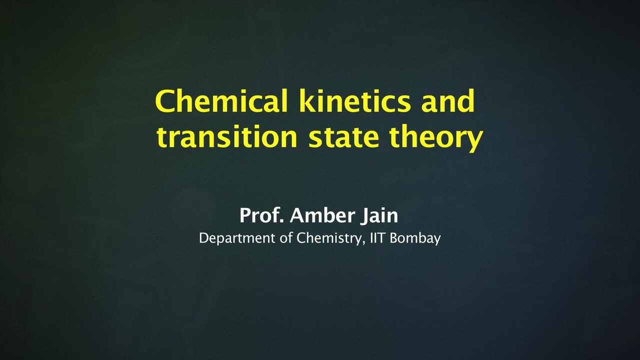 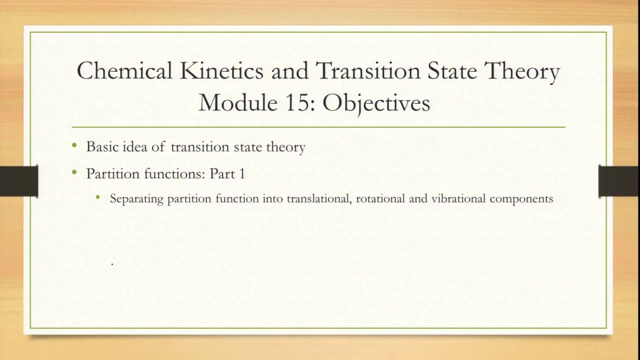 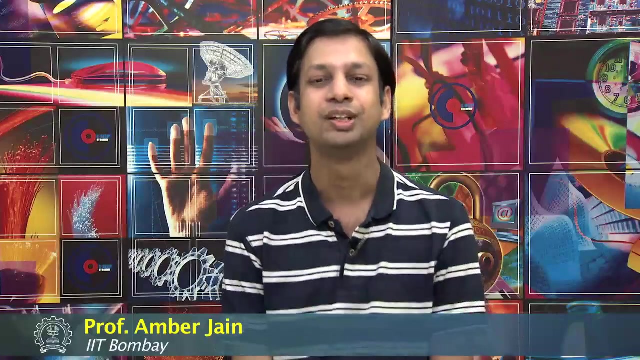 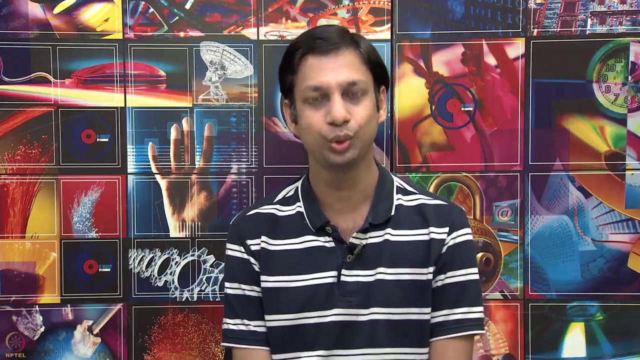 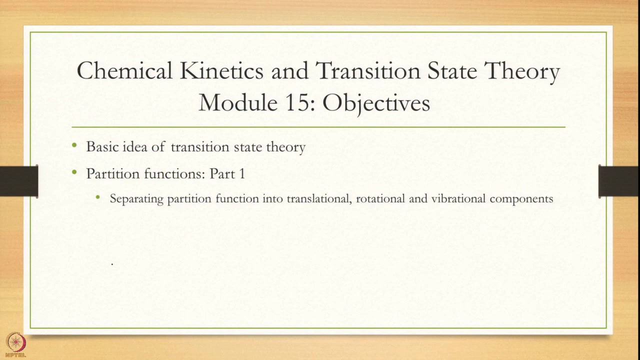 Hello and welcome to module 15 of Chemical Kinetics and Transition State Theory. Today we are going to start a new chapter. This course essentially focuses on two different theories: Kinetic Theory of Collisions and Transition State Theory. We have looked in some detail the 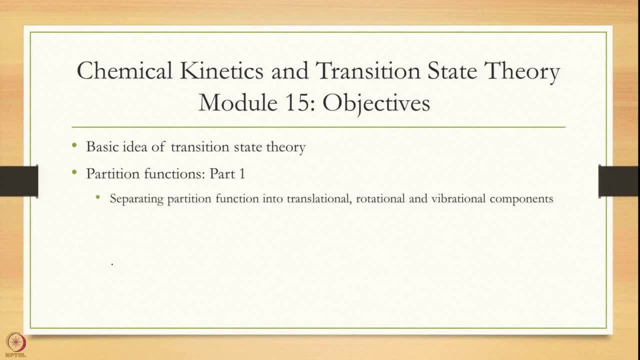 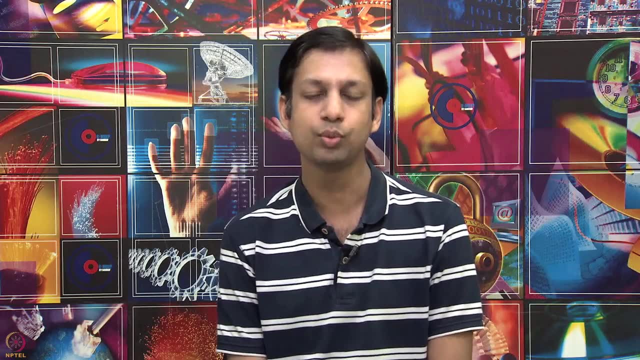 Kinetic Theory of Collisions. What we have also looked into is the limitations of Kinetic Theory of Collisions in the last module. So today we are going to build over more popular and more successful theory, which is called the Transition State Theory. Today we will 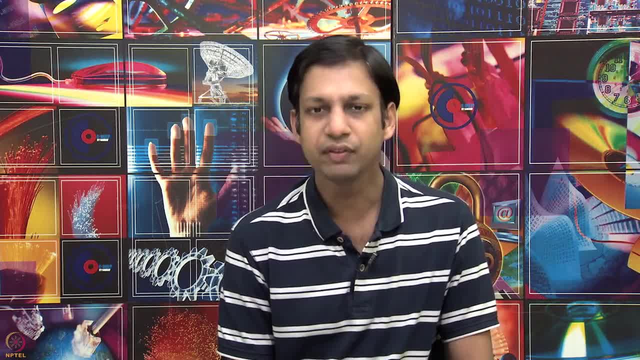 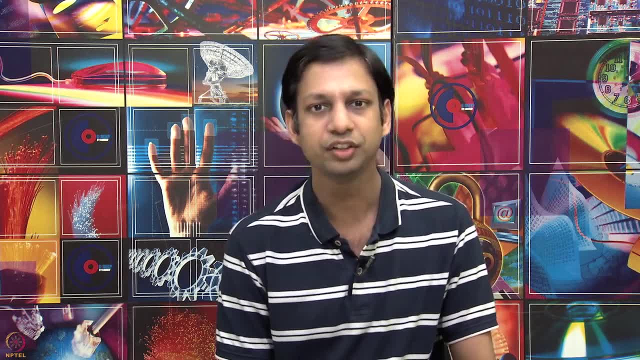 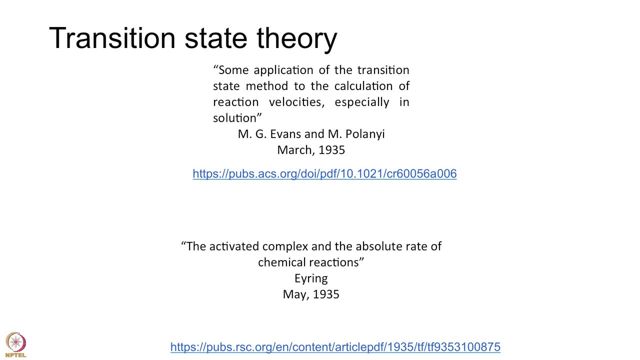 introduce the basic idea of Transition State Theory, and then we will have to take a little detour of statistical mechanics, particularly knowing partition functions. So let us start So. the Transition State Theory came about in 1935. There was a precursor to Transition. 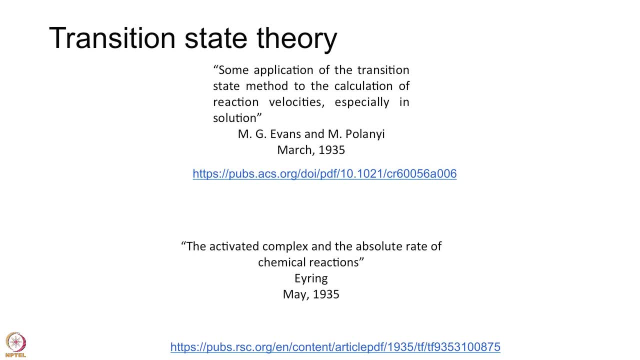 State Theory in 1932 by Wigner, very nice paper but it had missed a few important factors. In 1935, there were two papers, one by Evans and Poliani, March of 1935, some applications on the transition state method to the calculation of reaction velocities. So back in that day, 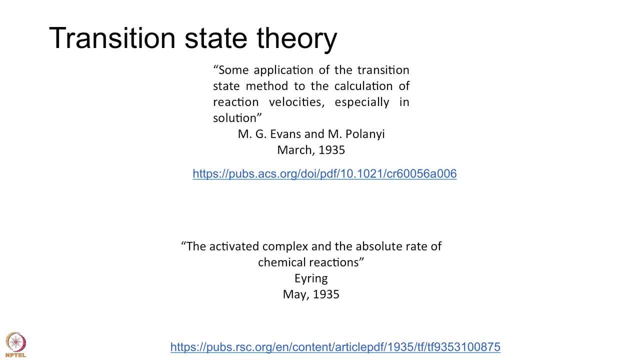 reaction velocity is the same as rate constant, And the second one was by Eyring, the activated complex and the absolute rate of chemical reactions, And the absolute rate again means rate constant. So these three people had essentially developed Transition State Theory. 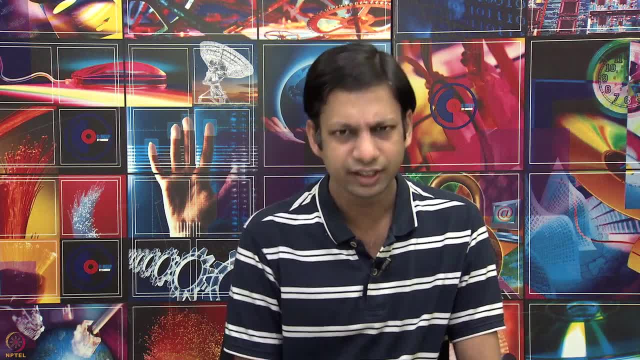 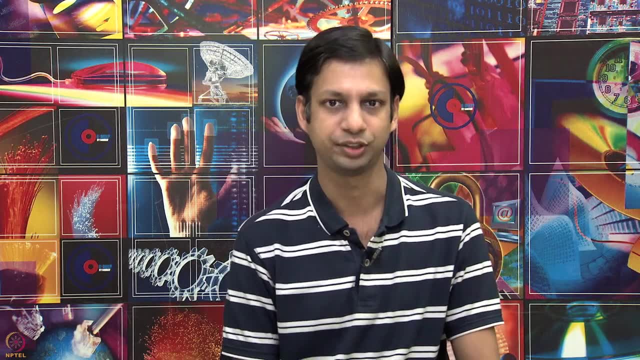 Both the papers developed very quickly, But they both had very similar theories. So the similar idea and combined together it is called transition state theory today. And, by the way, the formulas written in these papers are still used today. So in the next several 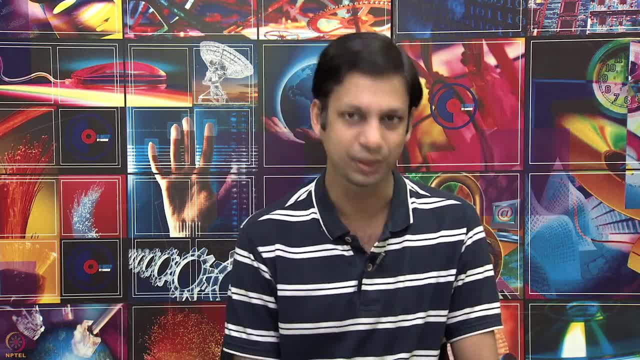 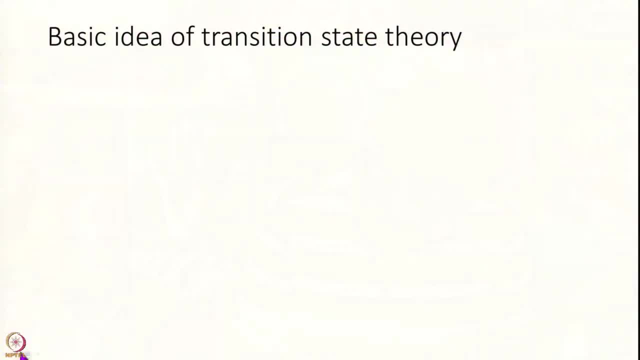 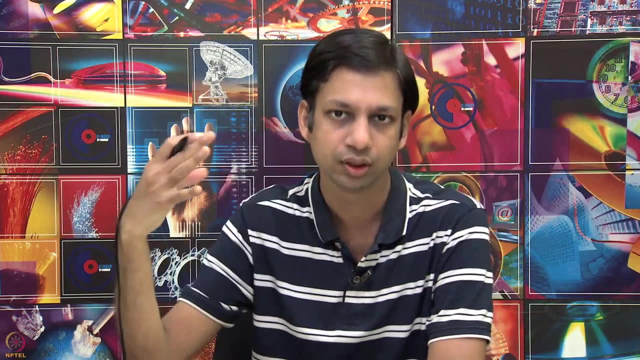 modules. we are going to understand what was developed by in these papers. So let us look at: what is the idea, what are we doing? So remember, in kinetic theory of collisions, what is really missing is the idea of chemical bonding, The whole chemistry. 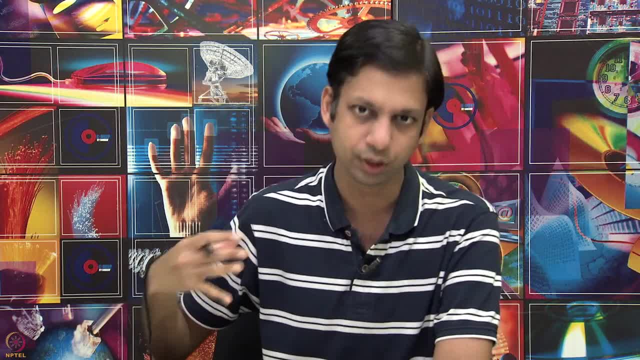 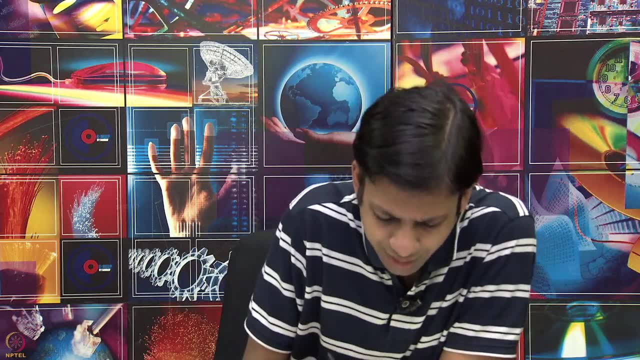 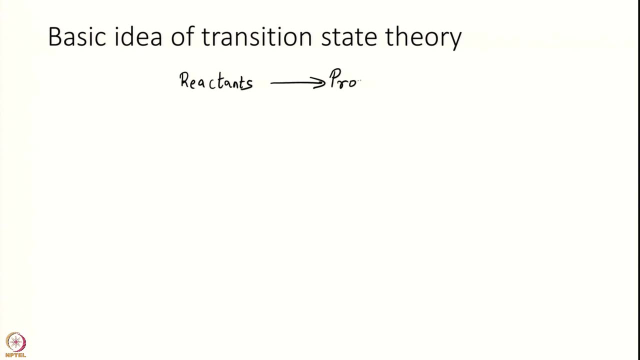 was missing. So we want to get that in into the picture and we are essentially going to use the intuition that Arrhenius had provided. So let us start. let us say I have some reactants going to some products. The most general reaction reactants can be a combination or it can be. 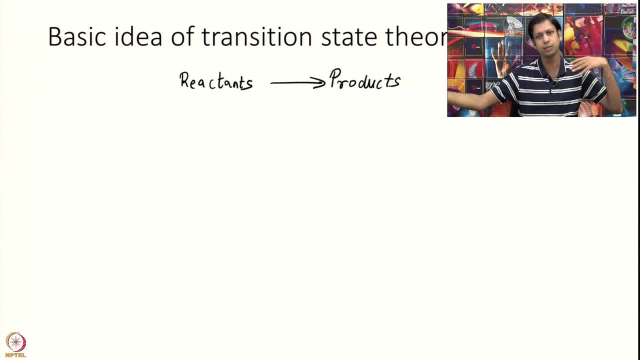 bimolecular, unimolecular, as any number of reactants to any number of products. So let me just write this in general as r going to p. I do not mean this to be unimolecular. when I write r, r can be a plus b, r can be a plus b plus c, some r And eventually what we want to find is the rate. 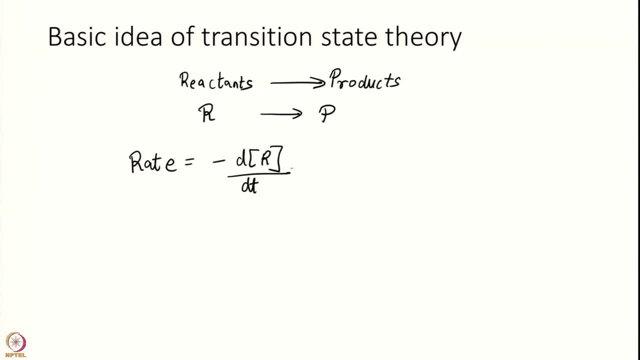 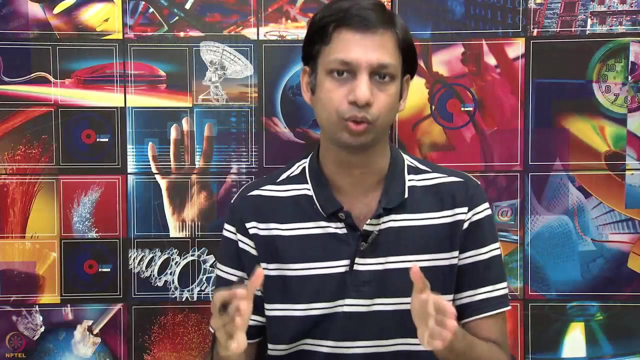 which, if you remember, is defined to be this: at constant volume. Please do note that in writing, this definition of rate, I am not assuming this step is elementary. This equation holds as long as volume is constant. So this rate is what I want to find and the postulate that transition state theory comes about. 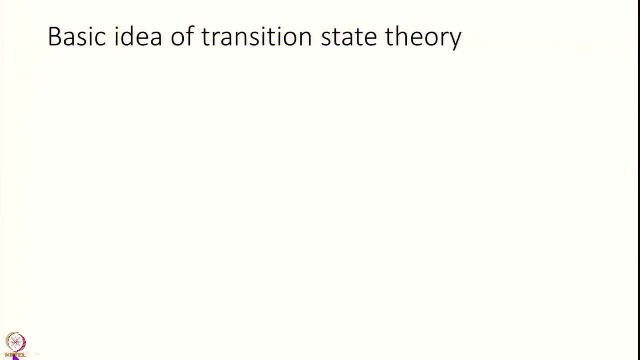 is the following: I have these reactants and I have these products, and we bring in the ideal of transition state that Arrhenius was talking about, And so I have a transition state in between, and the reaction between reactant and transition state is one at equilibrium. 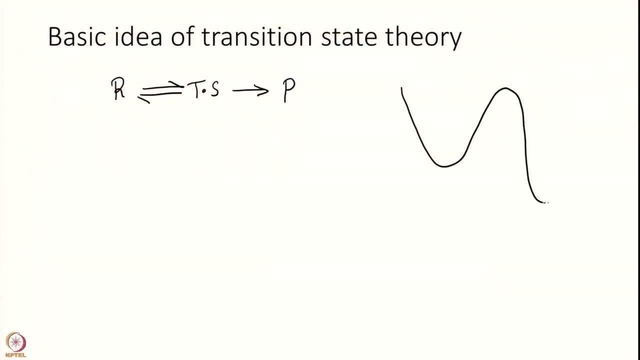 So pictorially, the idea is I am drawing a 1-D figure because that is easy to draw. I have some coordinate here. call it the reaction coordinate, if you will. some potential energy here. energy here, So this is reactants, this is products and in between, since the transition, 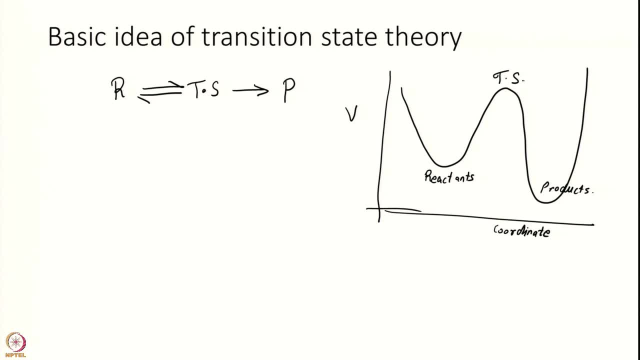 state- ok, So that is the main focus of transition state theory, the in between structure. So what we assume is that initially I am at reactants- ok, So I am initially here and I have an equilibrium with transition state. I am at thermal equilibrium with the transition state. 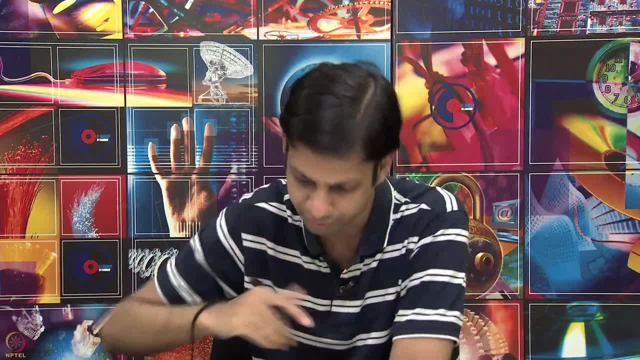 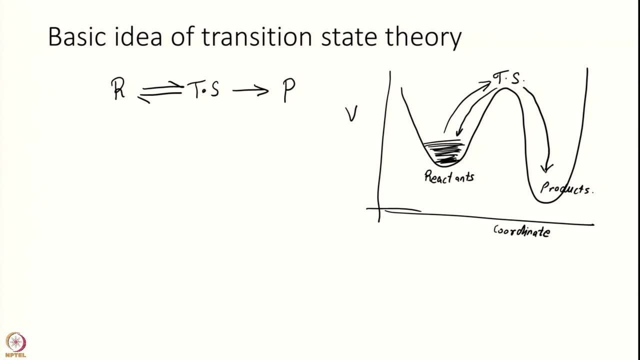 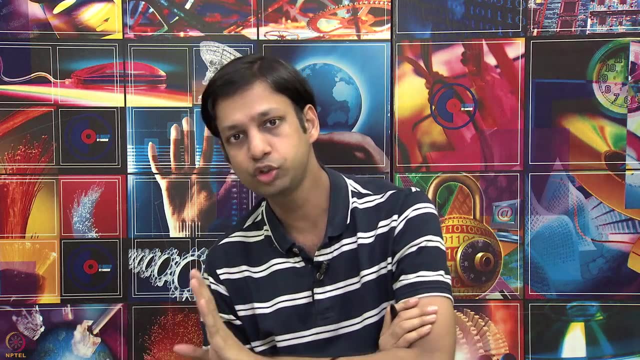 So reactants can go to transition state. transition state can come back to reactants, But transition state can also fall down to products, and one of the critical assumptions of transition state is that going from transition state to product is one way. So there is. 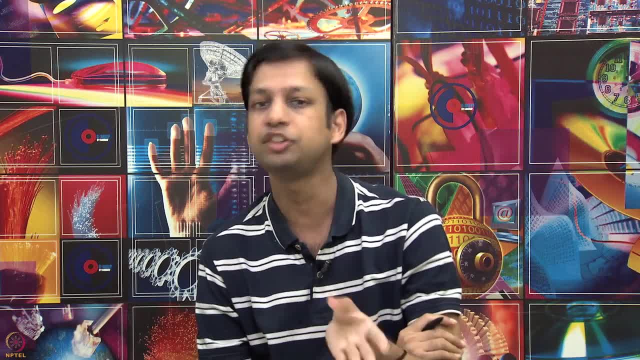 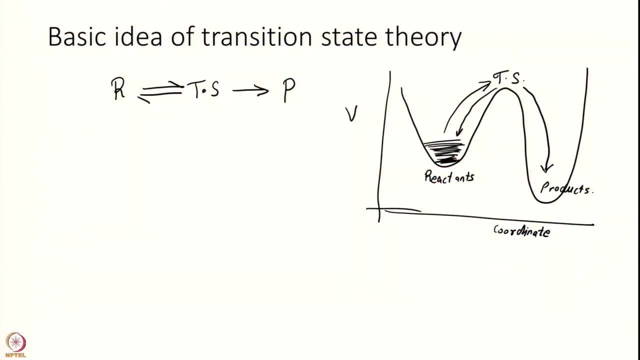 no equilibrium, no back reaction from product to transition state. It is one of the critical assumptions and we are going to do that. discuss these assumptions in great detail later on. ok, So let us think about this model. I have a k 1 here and a k minus 1 here, and I have a. 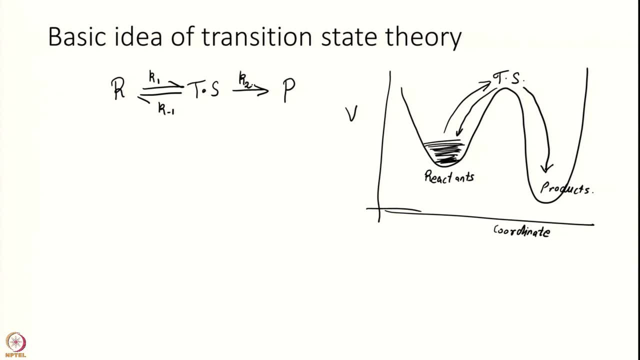 some k 2 here and all these steps are assumed to be elementary. So if I want to find the rate rate was dp over dt. but I can look at this elementary step. transition state going to product dp over dt will be equal to k 2 into concentration of transition state. ok, 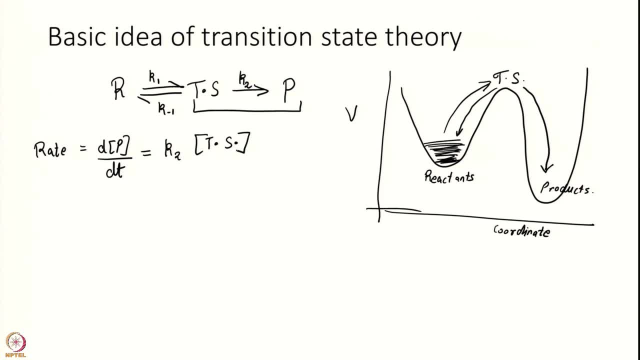 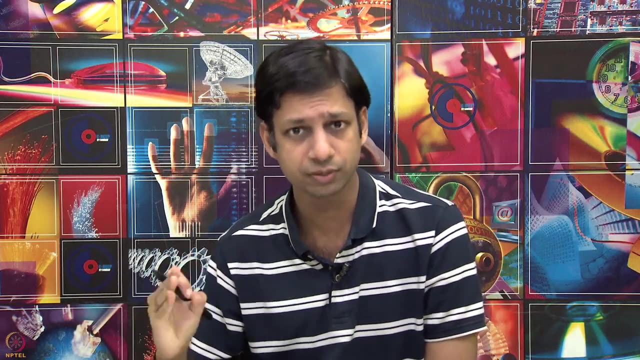 So that is how we write rate loss. or you can go back to our very first module, where we defined module 1 or module 2. ok, So the next thing we assume is that reactant and transition state are at thermal equilibrium, which means that the forward rate will be. 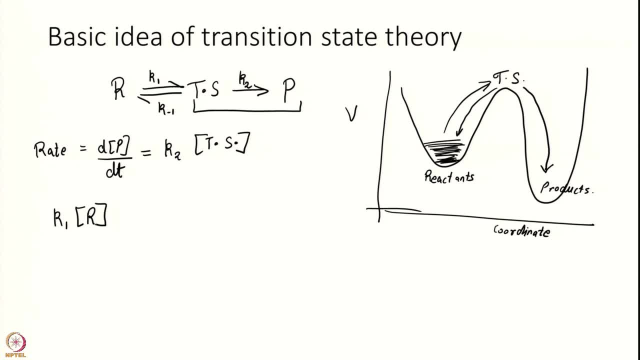 at k, 1 into r: ok, So this is r going to transition state. this rate is equal to the backwards rate, So this is forward rate, k minus 1 into transition state. So this is the backward rate. So at equilibrium, which is an assumption, ok, So we are making some assumptions to. 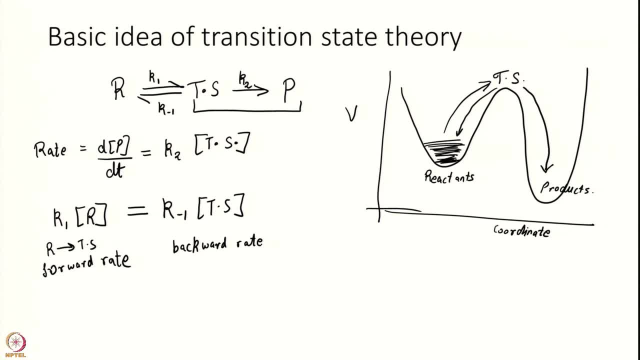 build our theory Is equal to this. So from this I derive: transition state concentration equal to k 1 over k minus 1 into r, and k 1 over k minus 1 is what we call as k equilibrium. ok, k equilibrium is. 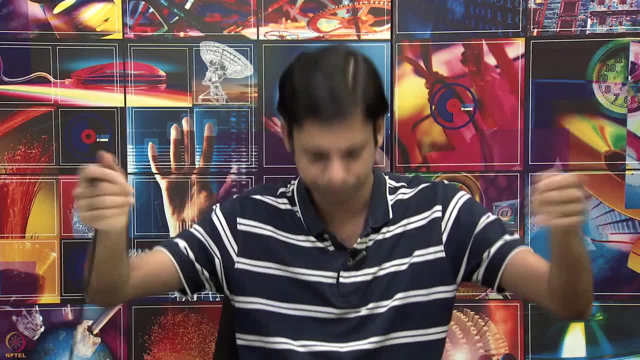 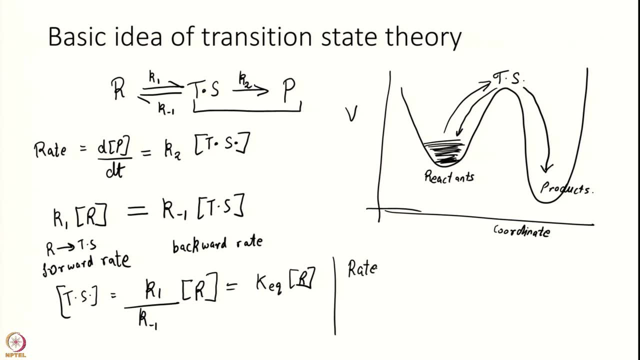 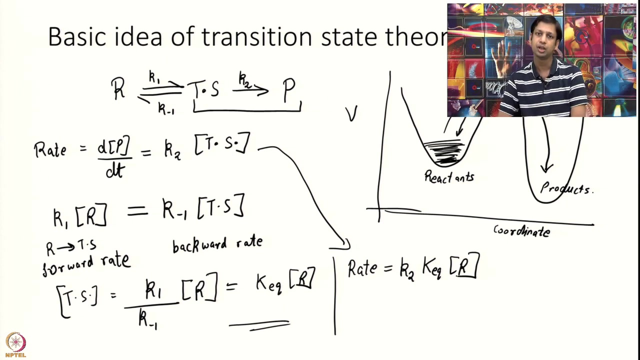 the equilibrium constant of r with transition state. So my rate is then. So I use this equation here: k 2 into concentration of transition state, which we have found here. ok, And so the after doing this basic analysis, making all these assumptions, what we have to do now is estimate k 2 and k equilibrium. 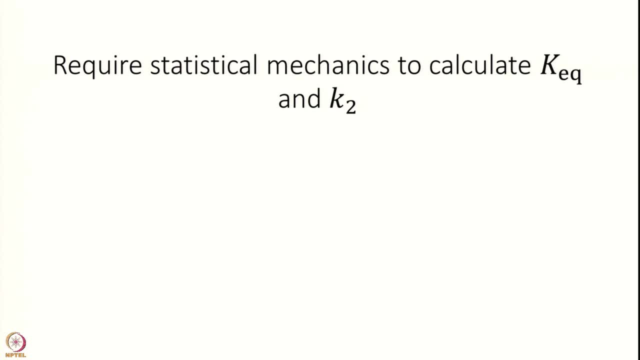 ok, So to calculate this k equilibrium and k 2, we require little bit of statistical mechanics. Without that we cannot actually calculate this. and as it turns out, this k equilibrium particularly is related to what is called a partition functions. ok, So these relations? 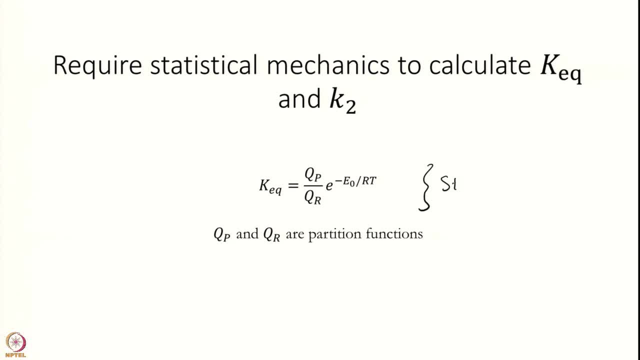 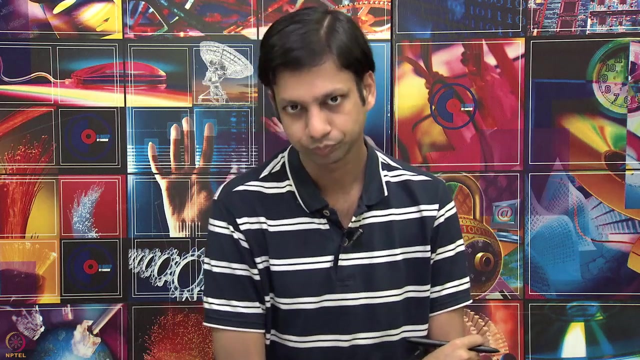 are very fundamental in statistical mechanics, and to understand these relations, we will need to study partition functions. So that is what we are going to do in today's and next module, And perhaps the next one as well- is understanding partition functions So that we can calculate this k equilibrium. 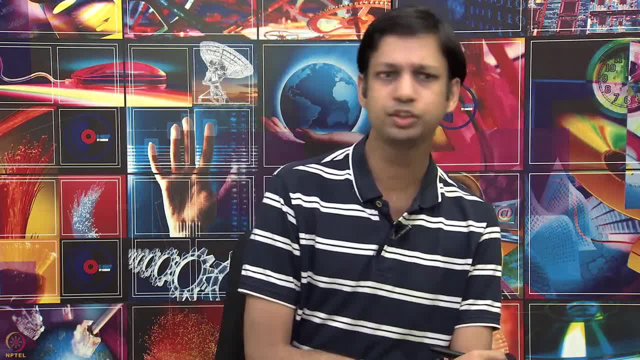 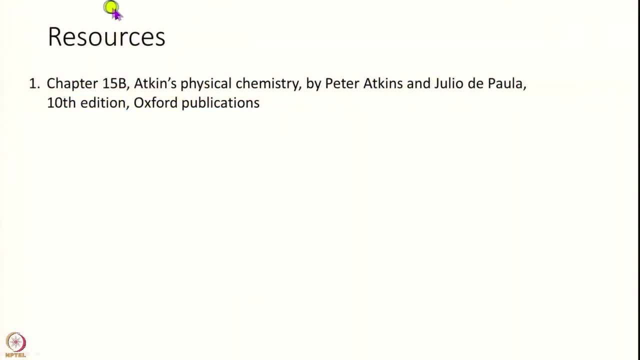 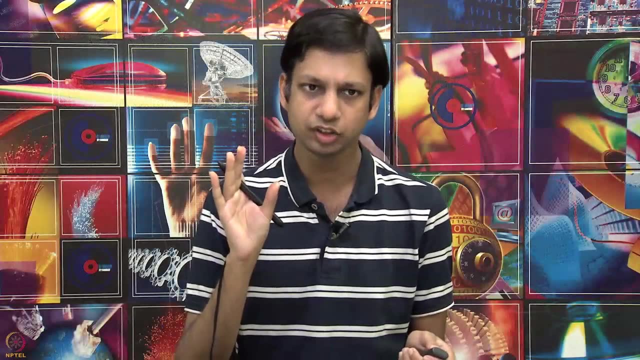 So this partition functions. you can read in the Atkins book: I have provided you this particular edition, 10th edition, chapter 15B. You have any other edition, please do not worry, you will be able to find this particular content in some other chapter number. The content: 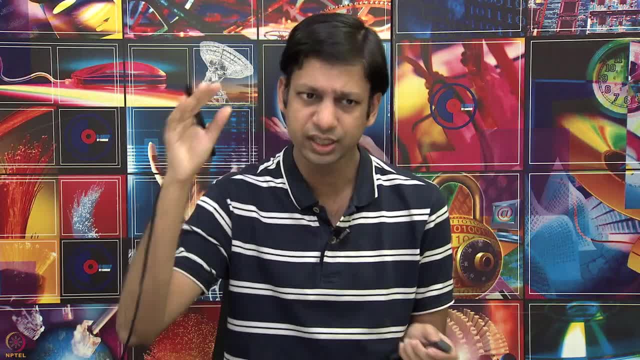 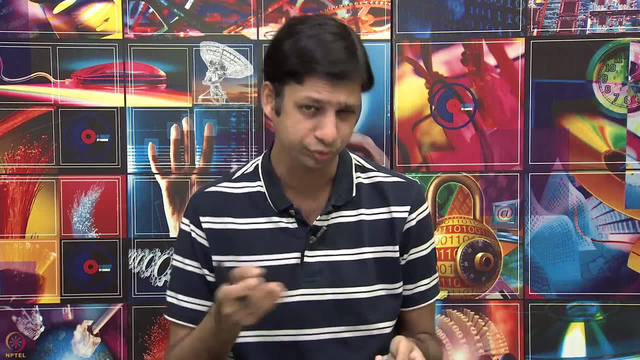 remains the same. the chapter number changes, So you do not have to spend more money in getting the 10th edition. You will be able to find it in any other edition. Of course, partition functions you can find in many other standard textbooks of statistical mechanics. 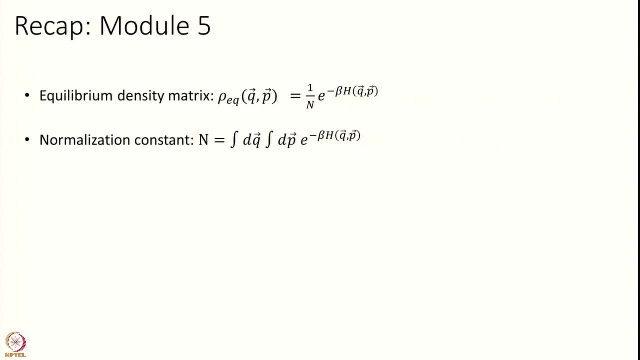 or even online. So we will recap something very old, Much ago, 10 modules ago, we derived something very fundamental: That at 10th edition, we can write a partition function, So we can write a partition function. That at 10th edition, we can write a partition function, So we can write a partition function. 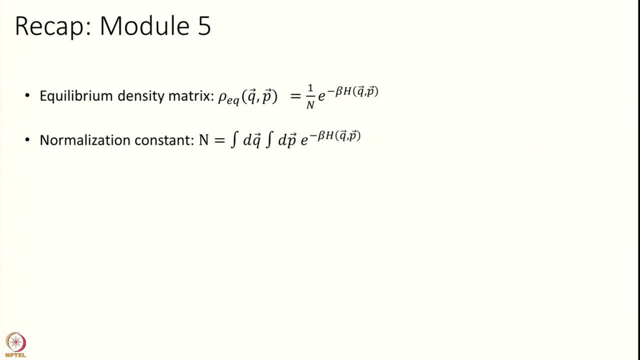 If we write it in 10th edition, we can write that a k equilibrium, the classical density matrix looks likethe 1 over n into e to the power of minus beta h, And my n, which is a normalization constant we showed, is equal to this. You can go back to this module where 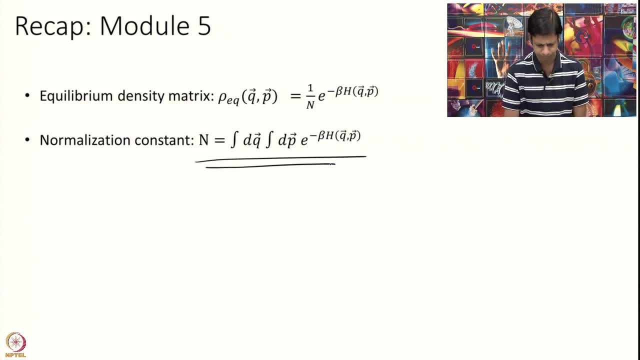 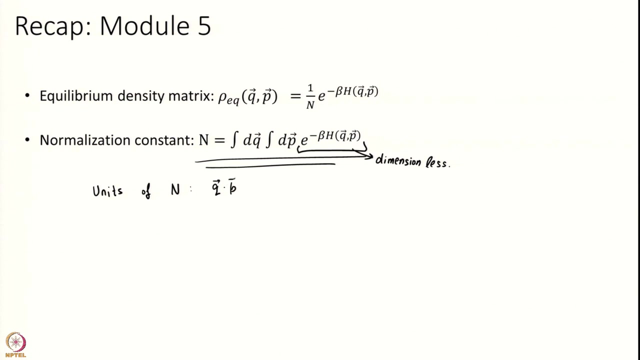 we have derived this partial derivation in phase space. We will build over it right now. What is the units of n? Well, it is. we see that this thing is dimensionless, it is an exponential. So the units of n is the same unit as q into p. ok, What is the dimension? 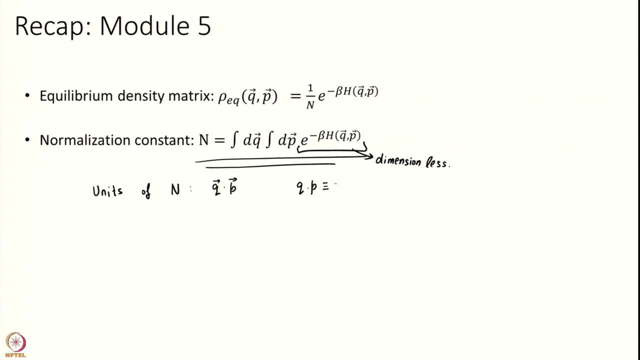 of 1 q into 1 p. that is equal to q is unit of length, So in SI units it is meter. p is momentum, which is kilogram meter per second. which is kilogram meter square per second. Does this unit remind you of any fundamental constant of nature? It should strike you something. 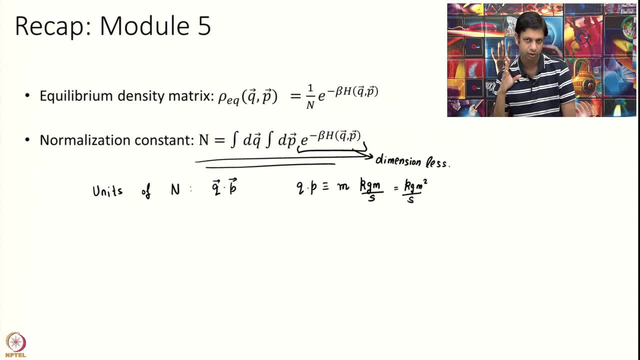 that is related to kilogram meter per square per second. If you guessed h or h is equal to h bar, you are exactly right. This is the same units of h, the Planck's constant. ok, So q dot p. this is 3 n. q dot p. ok, So q is a 3 n dimensional vector where n is the. 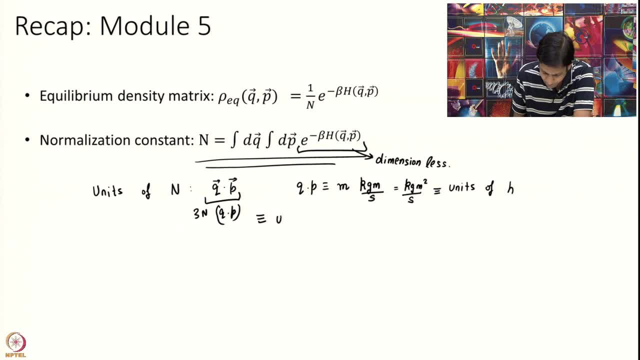 number of particles. So this thing is the same units as h to the power of 3 n. Each q dot p gives me 1 n, So I have 3 n q dot p, So I get h to the power of 3 n. So the first thing we do, actually, 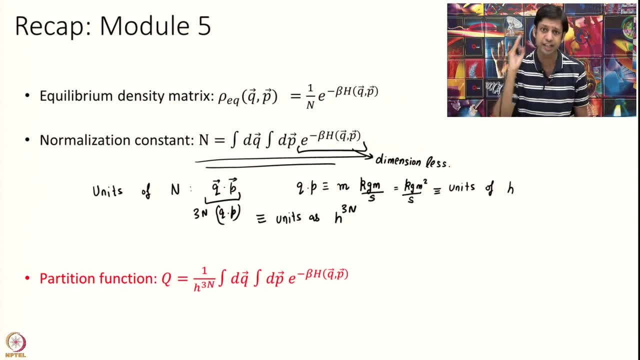 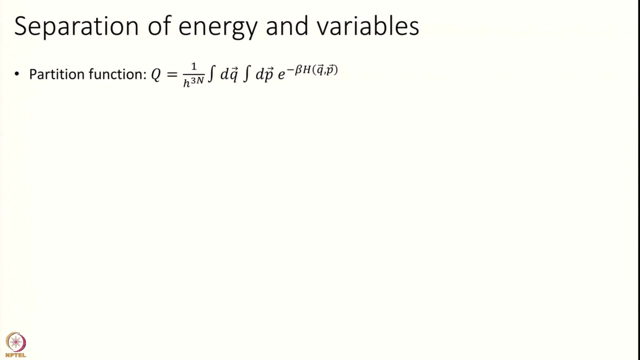 is to define a partition function, q, which is dimensionless. So we take this n and divide by h to the power of 3, n. ok, So this thing is dimensionless. ok, So this thing is dimensionless. ok, So we start with this partition function and what we do is this: by itself is very large. 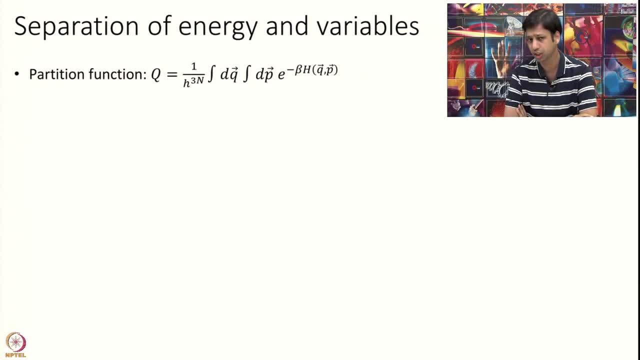 very, very complex to calculate. This is a 3, 6 n dimensional integral. I have 3 n q's. I have 3 n p's. I do not want to do this integral. I do not know how to do this integral. 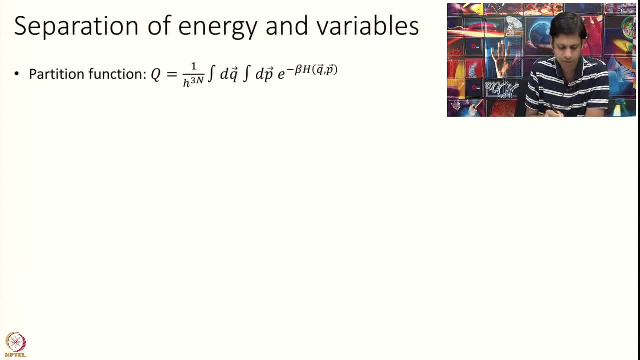 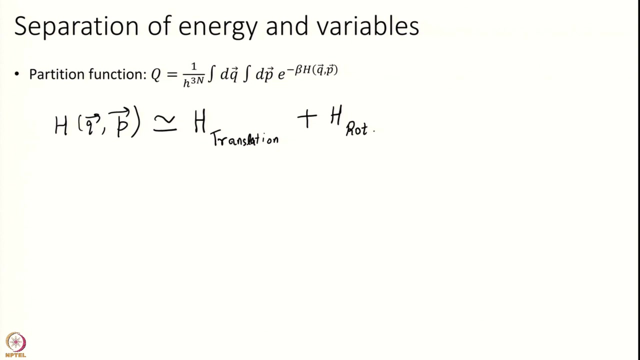 We will simplify our life. What we do is we note one important property of the Hamiltonian. This to a good approximation, for most problems can be separated into Hamiltonian of translation, plus Hamiltonian of rotation, plus Hamiltonian of vibration. ok, Once we bring in quantum. 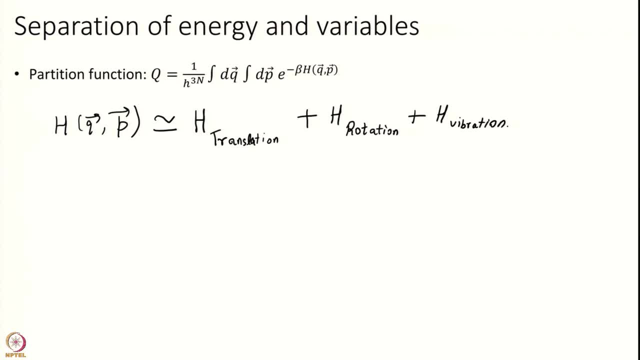 mechanics. we will also have an electronic part, but that I am not writing right now, So this is an approximation. This is not always separable. translational part can always be separated, but rotation and vibration in principle can be mixed. but we will make the 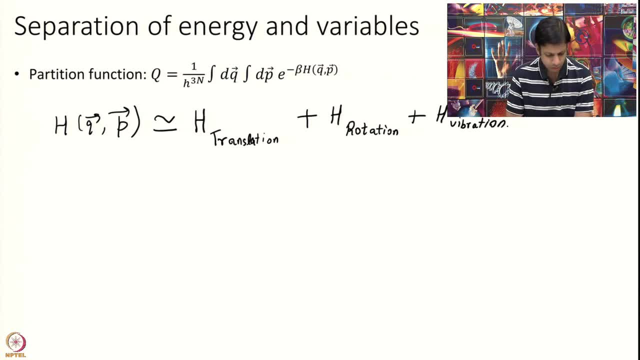 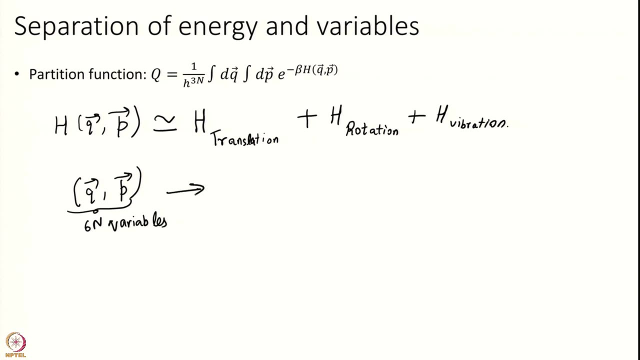 simplification for now, for this course. ok, How do we make this simplification? let us say we will have to provide one more thing: the q comma, p, These are 6 n variables. So this itself is partitioned into translational, which is nothing but center of mass. so these 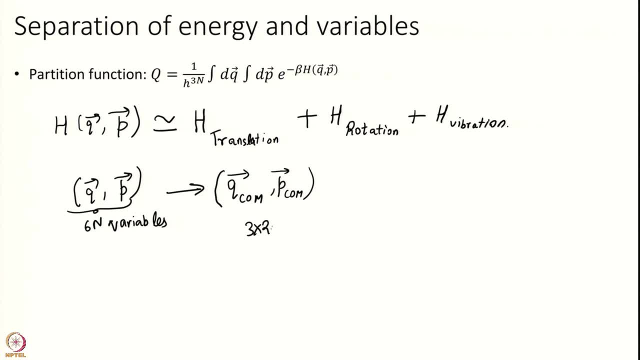 are 3 coordinates, 3 into 2, 6 variables, so the entire center of mass of the my molecule. okay, so x, y z of center of mass and p, x, p y, p z of my center of mass. plus I have 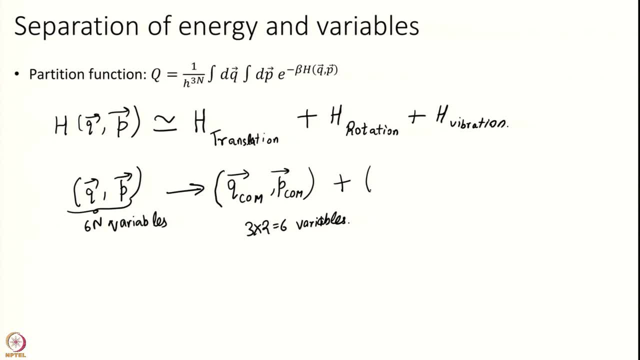 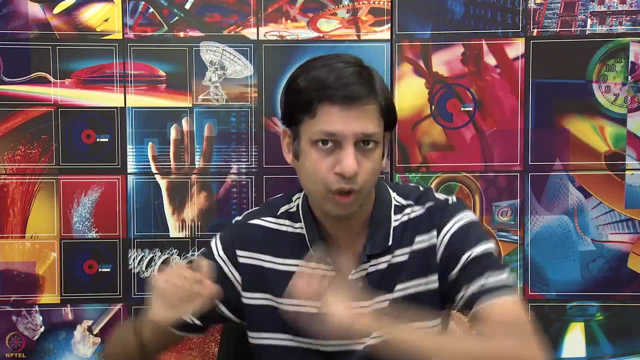 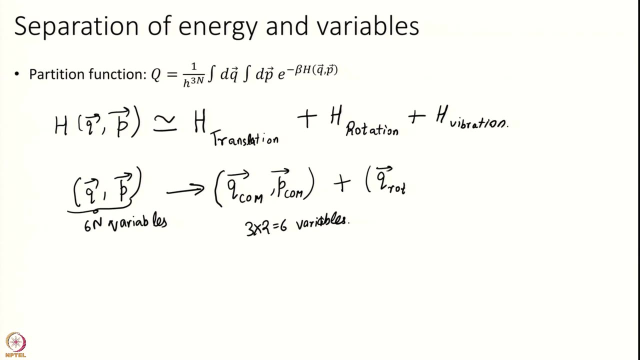 also coordinates and momenta describing rotation. so that tells me how the molecule is oriented and what is the angular momentum of my molecule, of the overall molecule, okay, how it is rotating around. So I have q rotation, p rotation, x, y, z of center of mass and p x, p, y, p z of center. 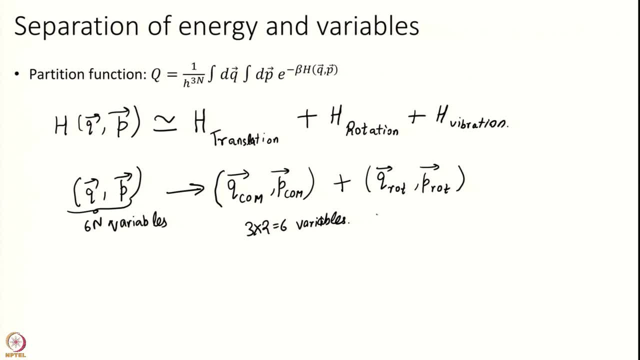 of mass. So this is a slightly more complex. for linear molecule there are only 2 rotations possible. we will discuss this in a moment. so 2 into 2, 2 angles and 2 corresponding angular momenta, so 4 variables. 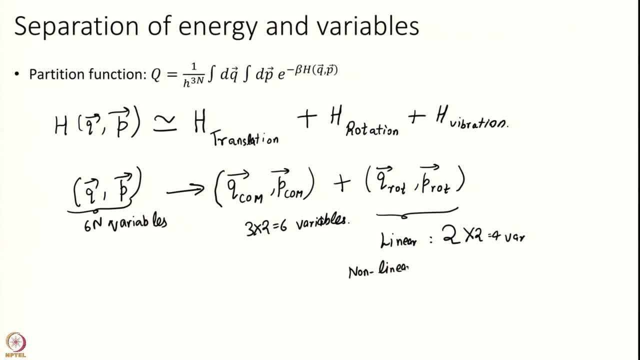 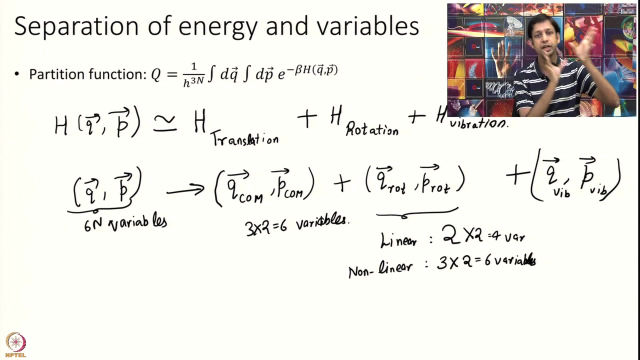 For non-linear. we will discuss this in the next slide. please do not worry. we can have 3 possible rotations And finally we have q p of vibrations. okay, so not only do we separate out the Hamiltonian, we have also separated outer coordinates and momenta. 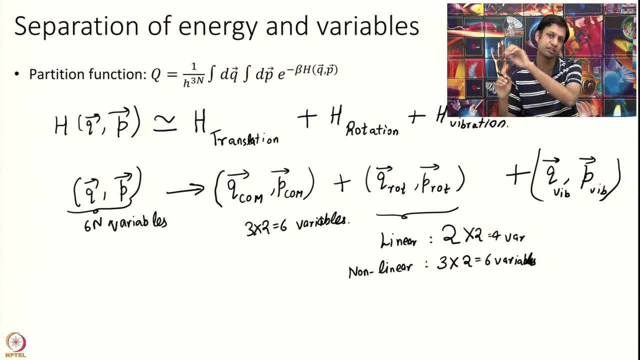 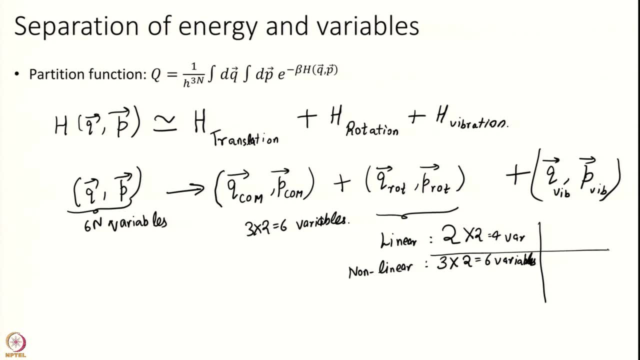 We have coordinates describing translation, coordinates describing rotation and coordinates describing vibrations. So again for linear You vibrations will essentially become 6 n minus 4, remember the total has to be 6 n. I had 6 n variables here. I should have 6 n variables on the right. 6 have been taken. 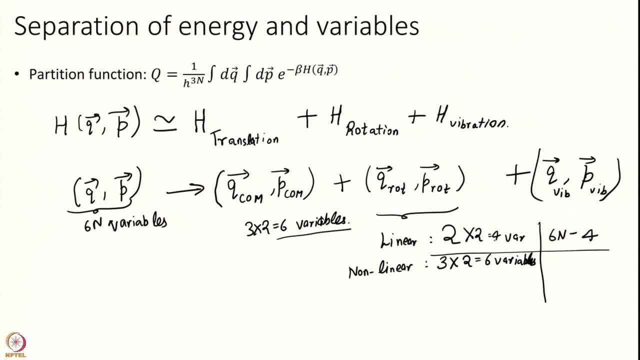 for translation, 4 for rotation. so I am sorry, my maths should become 6 n minus 10, for linear, okay, And for non-linear this will become 6: n minus 6 plus 6 is 12 minus 12, okay. 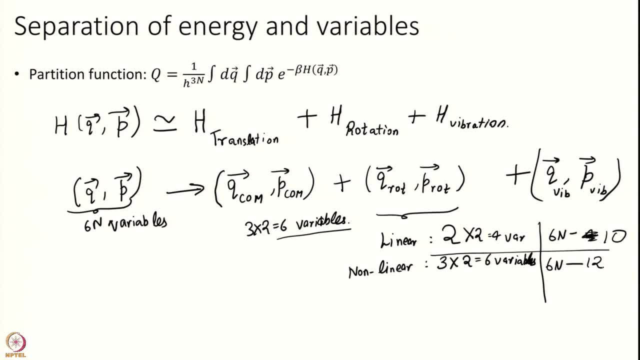 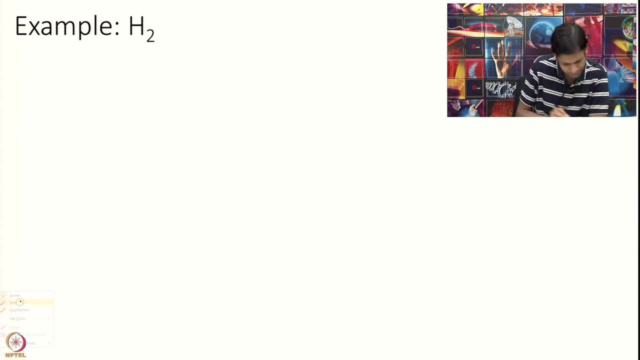 So I will have 6 n minus 10 vibrations, vibrational degrees of freedom- for linear molecules and 6 n minus 12 for non-linear. so let us look at an example. okay, things will become clearer. So let us start with a very simple linear molecule: H 2.. 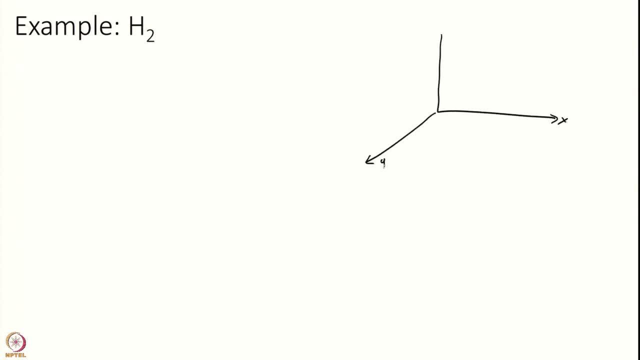 So let me just draw x, y, z and let us say I have some H 2 molecule oriented somewhere here. okay, So I have x 1, y 1, z 1 of the first and x 2, y 2 and z 2 of the second. hydrogen, yeah. 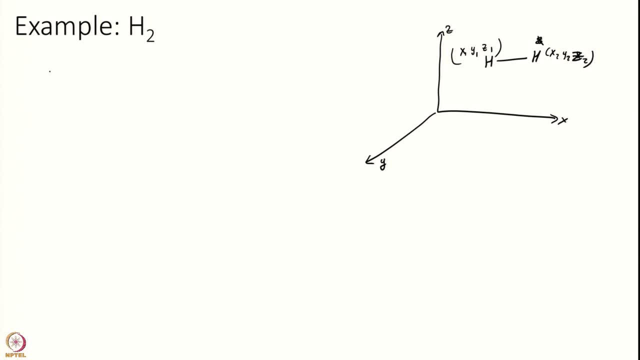 So I have 6 coordinates, Which is basically x 1, y 1, z 1, x 2, y 2, z 2, and we transform this into three center of mass. So we find a center of mass here, three center of mass coordinates. 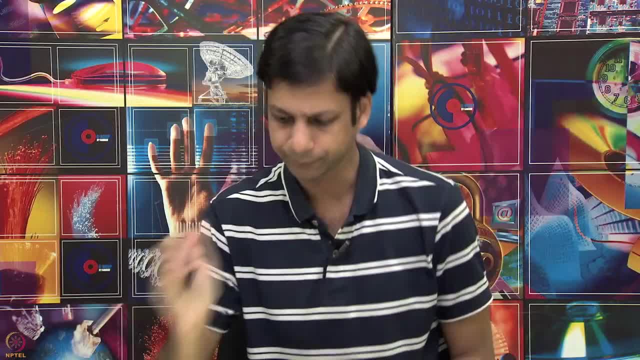 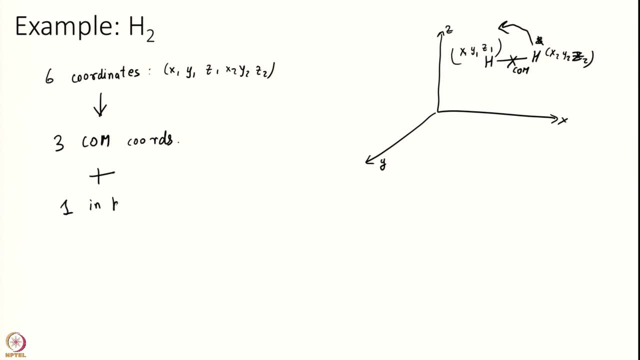 Now this molecule can rotate in two ways. One is this rotation in place, One in plane rotation plus one out of plane rotation. So for this molecule, I have to tell you theta and phi. essentially is what I am saying. You give me center of mass and you give me how the molecule is oriented in space, which? 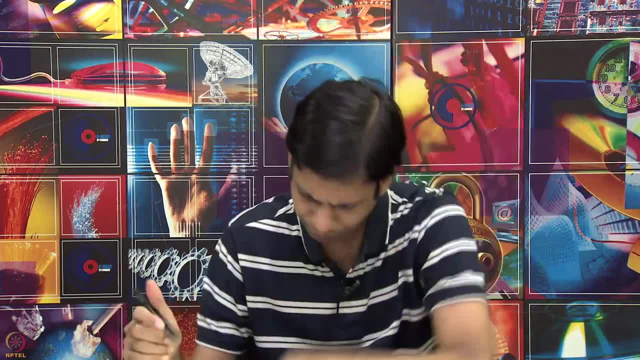 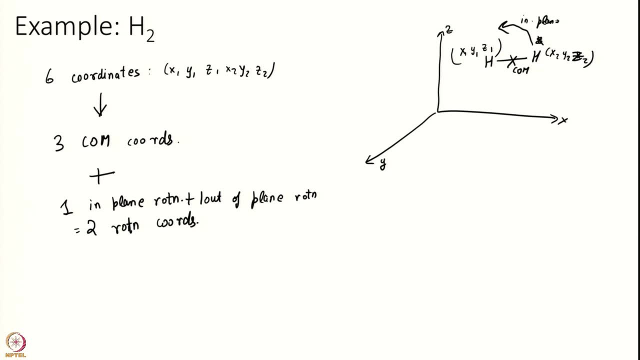 can be described? It can be described by theta and phi right. So for a linear molecule only two are enough. So one is in plane rotation and the other is. imagine this H 2 coming out of plane like this. So it is a hard thing to draw, but you can imagine something like this and this H is. 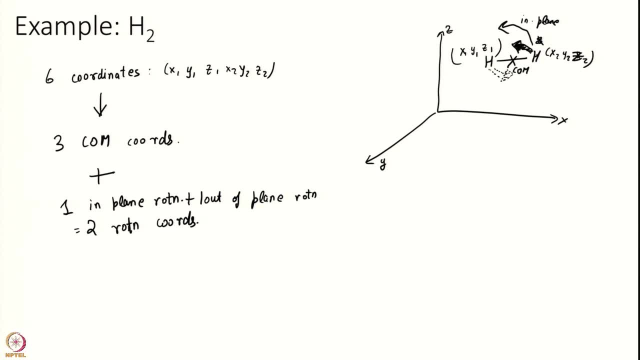 going under the plane, something like this. So the whole thing is rotating around like this, okay, And plus I have one vibration, H 2 can have only one vibration, which is this length. let me call this x. So you see I have a total of six: three center of mass, two rotation, one vibration. 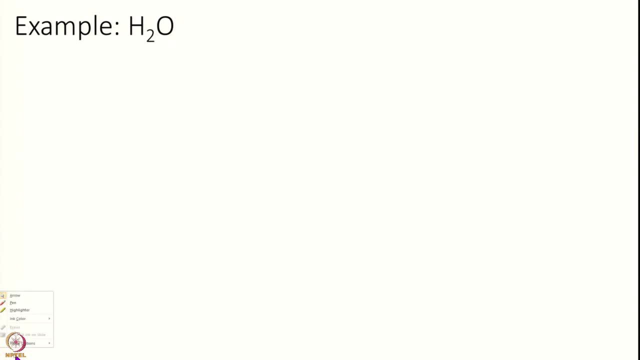 Let us look at a slightly more complex example which is non-linear. Let us look at water. So I have some orientation of water sitting here. Again, I have x, y, z. So now I have nine total coordinates: x 1, y 1, z 1 of hydrogen. x 1, y 1, z 1 of the second hydrogen, x 2,, x 3, y 3, z 3 of. 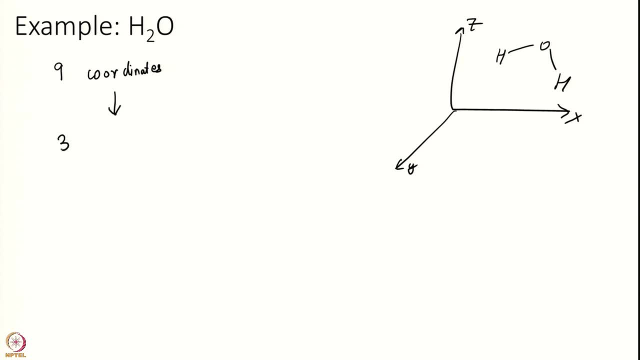 the oxygen. So again, I will always get three: center of mass. So wherever the center of mass lies, plus this time, I will have three rotations. why? Because you also have to describe how the water itself is oriented. So theta and phi tells me the overall structure. but beyond that as well, the molecule has internal 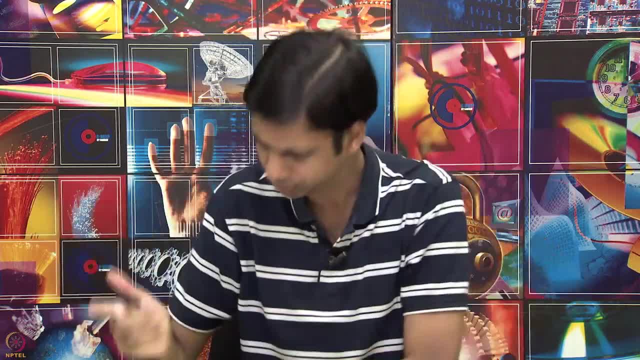 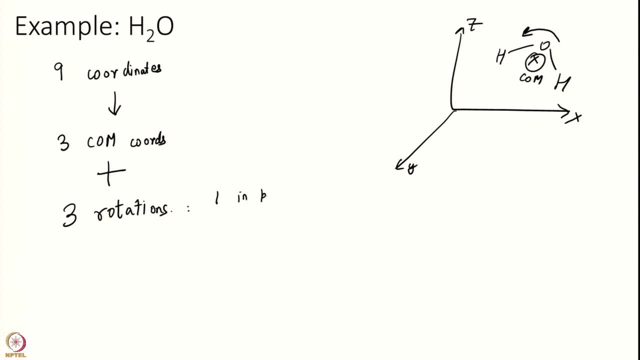 structure. So I can have one more degree of freedom. More physically, essentially, you have one in plane and two out of plane, So I can rotate the whole molecule in this manner. But I can also rotate the whole molecule in this manner. 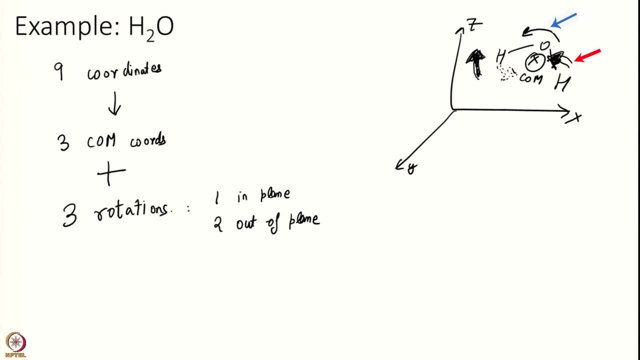 So one is in the plane, one is out of the plane like this, and I can also rotate it like this, So I have three possible rotations For H 2. this was not possible because your H 2 is rotating around the one axis. 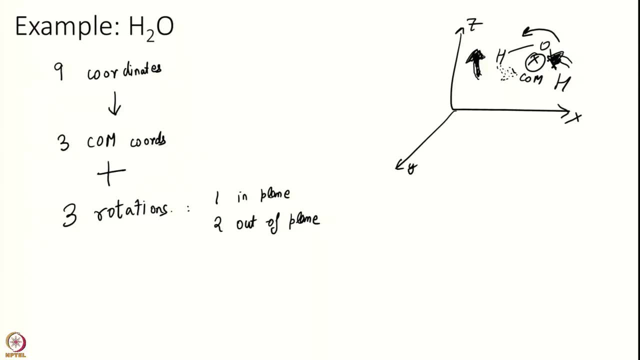 It is, yeah, so it that does not rotate at all. So that is the issue. And I have three vibrations, So for water I can have this stretch x 1, I have this stretch x 2 and finally I have the angle theta. ok, 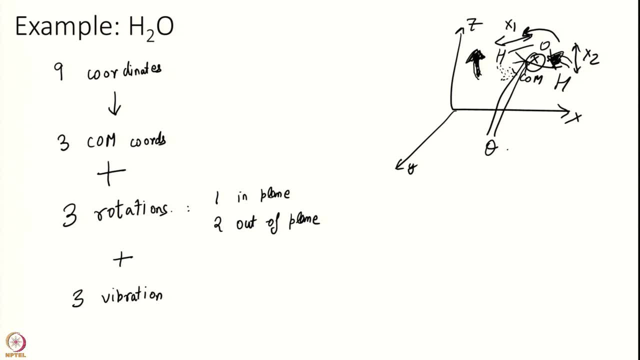 So I have three vibrations possible. So the mass will always work out. ok, So we have separated the energy. Let me just tell you a little bit more. So the mass will always work out. So the translational energy is essentially that of center of mass. ok, 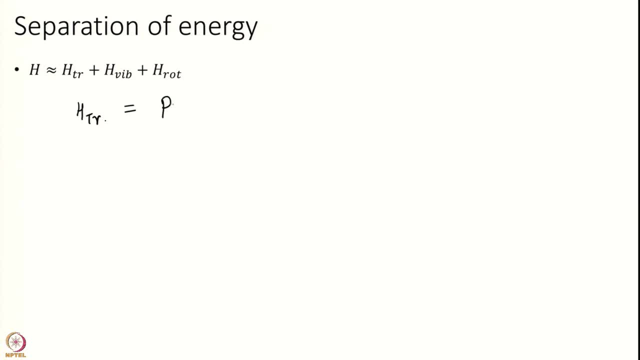 So this basically looks like momentum of center of mass, square divided by 2 m, where m is the sum of all masses, So m is the sum of all atoms. sum of sorry masses, So m is the sum of all atoms. 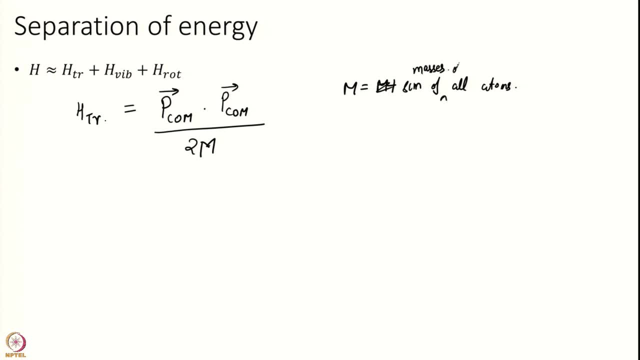 So m is the sum of all masses, So m is the sum of all atoms. So that is your translational energy. just the kinetic energy of your center of mass Rotation gets a little bit more complex. So I will not write the complex descriptions here, which is not necessary for this course. 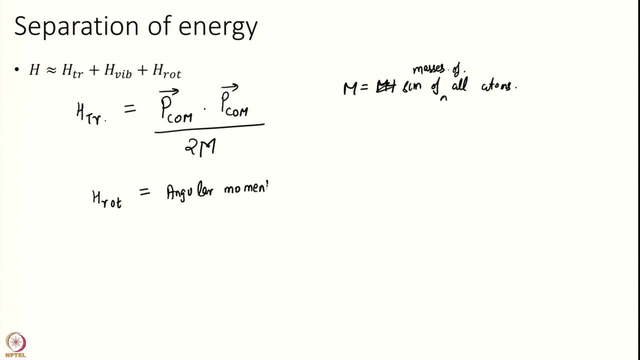 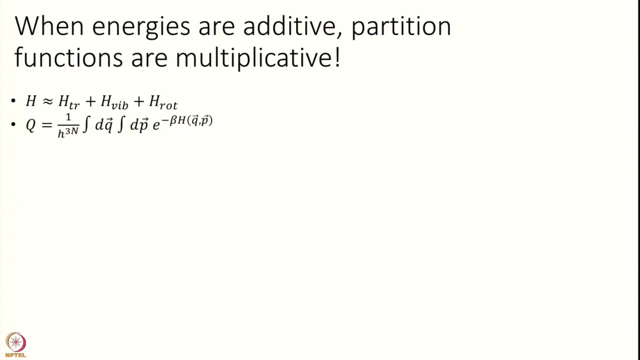 This, essentially, is the angular momentum, which is like L square over 2: I and, finally, is the vibration. 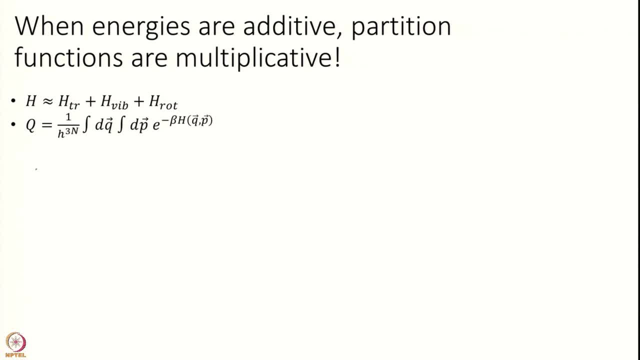 And let us put the separation of variable and the separation of Hamiltonian here. So remember, my q and p are now separated out, So I will write integral of d, q, dp in terms of a, q and p of translational rotational. 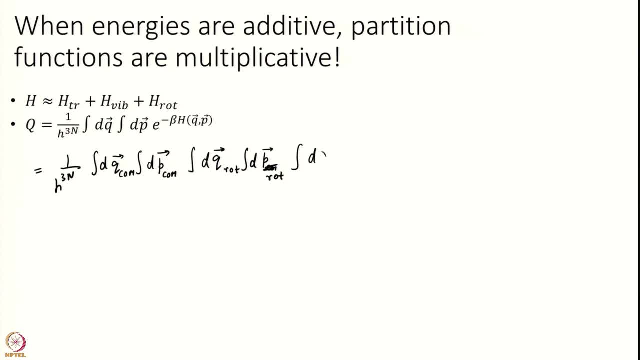 sorry, and vibrational and vibrational and Hamiltonian also I am separating out. 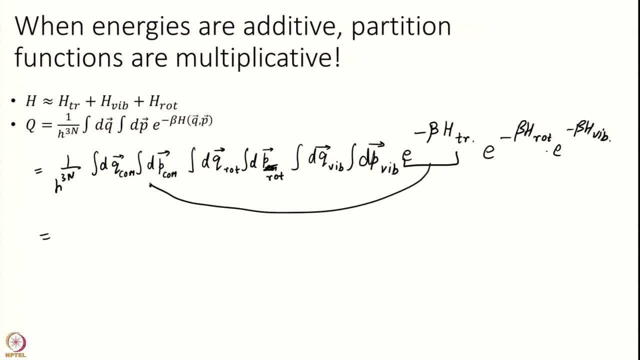 And then what we do is we? this depends only on center of mass, and this depends on this, and this depends on this. So I can write this as: 1 over h cube, dq, center of mass, dp, center of mass, e to the power of minus beta, h translation: 1 over h square for linear and h cube for non-linear. you understand? 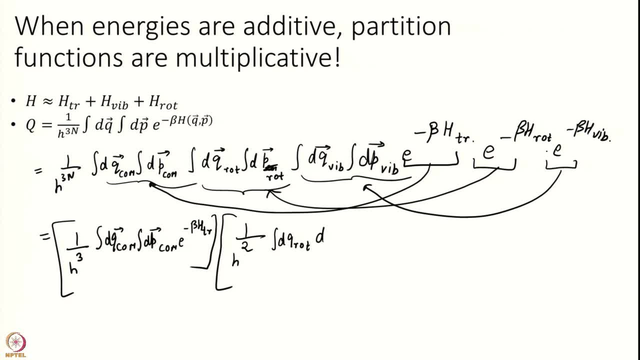 that now, So it does not matter. and finally, vibrations. and depending on linear or non-linear, I will have 1 over h to the power of 6 n minus 5, sorry, 3 n minus 5 or 3 n minus 6..